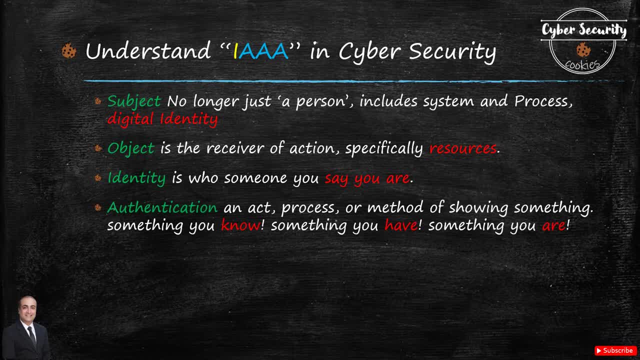 An authentication, on the other hand, is claiming your identity. How we will do it? It will be using something you know, or something you have, or something you are. We have few more slides coming, so let's hold on to that for now and move to the next concept of Authorization. 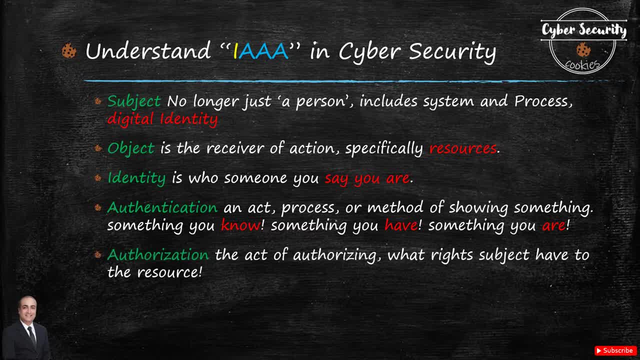 Authorization is the right of a subject holding an identity on an object. So if you are an owner of the house, you can enter all the rooms, But your friends have limited access. In case of a system, if you have access to a file, you have a, read, write, modify permission, but your co-workers only have read only. 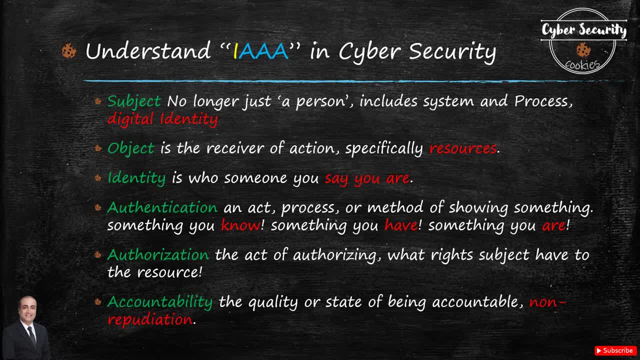 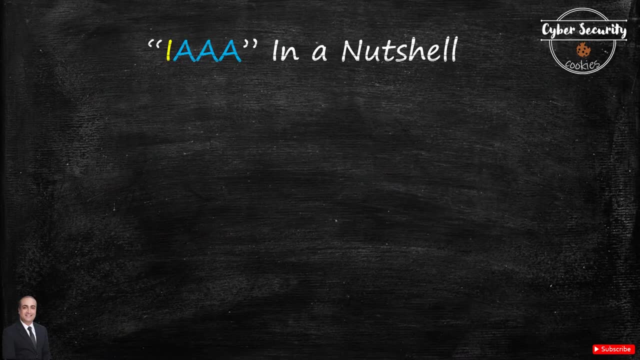 Accountability, on the other hand, is useful for non-repudiation. That means you cannot deny your actions. Let me take you to the next section and elaborate more about all of these. So IAAA in a nutshell. So, as we mentioned about subject: example users that might need access to an object, example databases, files, folders or emails. 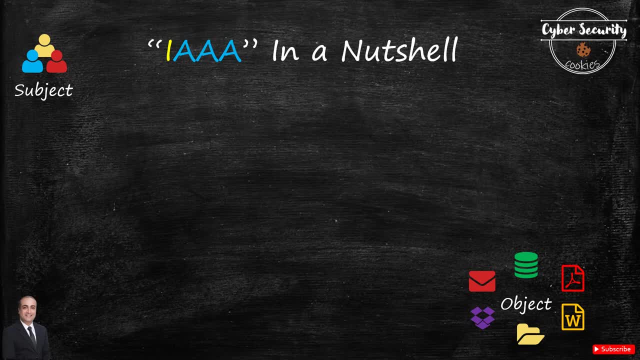 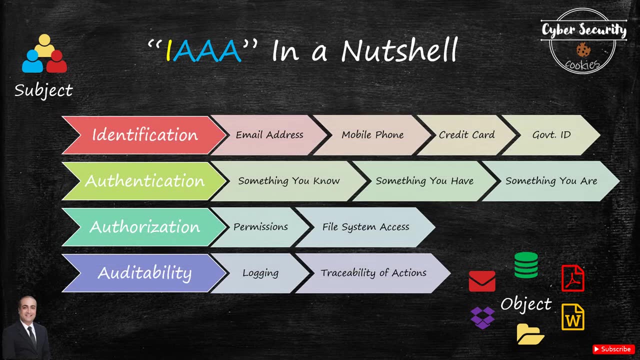 Or I give you a real-time example. Let's say you want to access a website And a website doesn't know on what basis they provide you access. Your email address will be your identity That system understands, as you used at the time of registration. 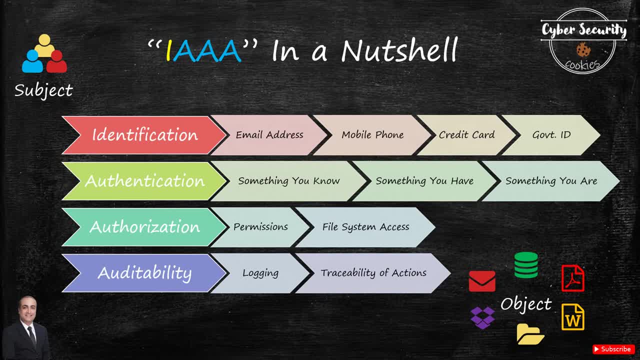 And there are different levels of identity that are provided And they are categorized into different levels, from 1 to 4.. So level 1 will be an email address. A level 2 can be a mobile phone. It can also include a credit card as a level 3.. 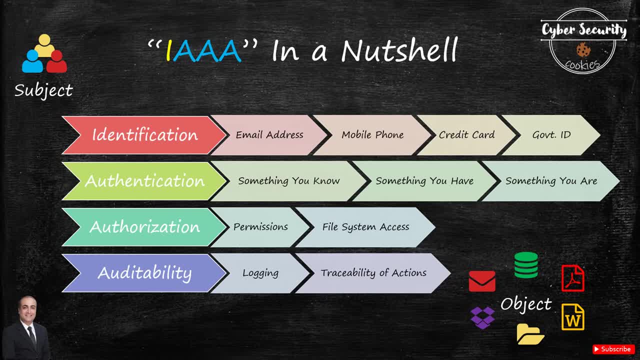 And a level 4 can be a government identity. So providing an email address is something- We say who we are. Once identified, we need to authenticate and prove our identity. You put a password or a PIN. That is something you know.